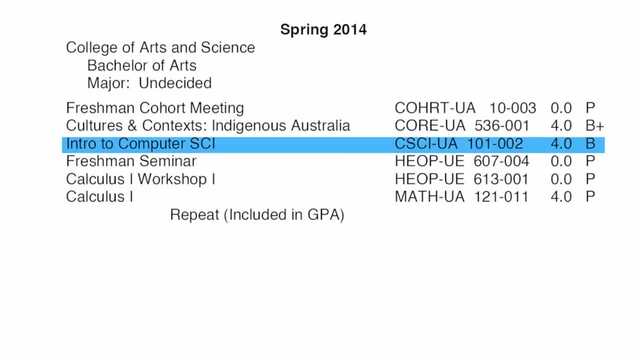 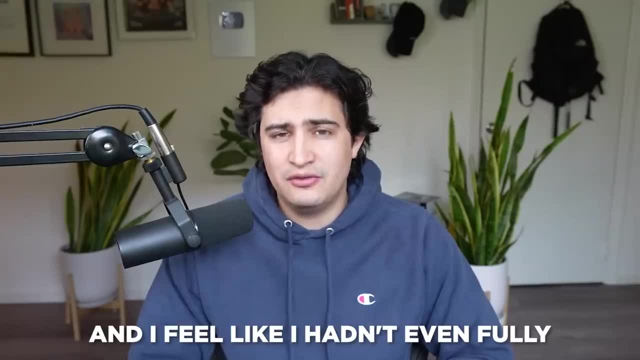 time for me to take my next computer science class, Intro to object-oriented programming, during my spring semester. I was actually worried about this class because during it I'd be learning a new language- Java- and I feel like I hadn't even fully understood Python yet. Luckily for me. 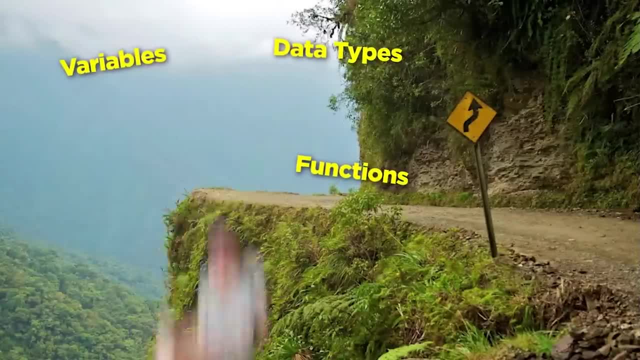 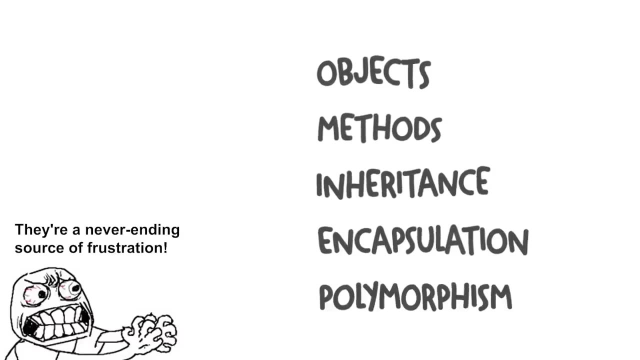 we did approximately zero review of all the underlying topics and jumped straight into object-oriented programming. We learned about topics like objects, methods, inheritance, encapsulation and polymorphism, And while it took me a while to get up to speed, I was slowly able. 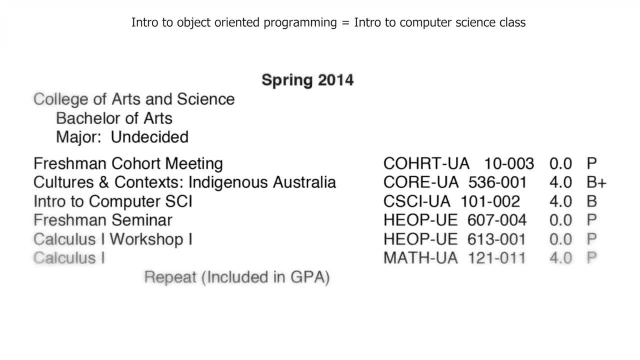 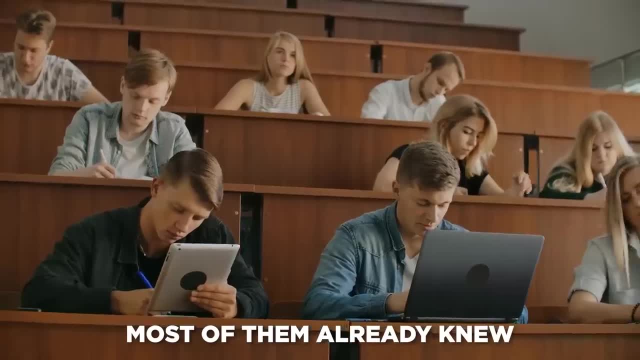 to relearn all my first semester of coding and squeak by my intro to object-oriented class with something around a B as a grade. Tons of other students in the class could pick up things way faster than I could process them. Most of them already knew how to code and could therefore 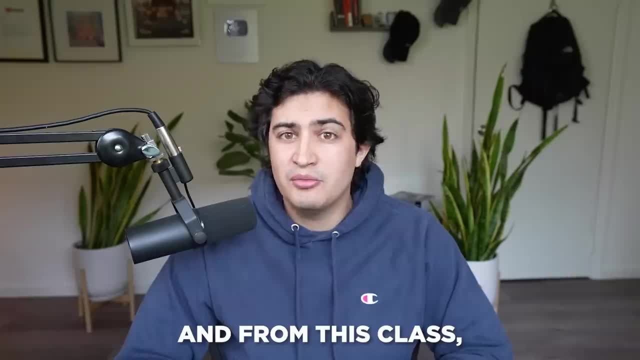 skip the Python class that I was required to take the previous semester, And from this class I learned my second lesson, which was that I liked programming but I really wasn't very good at it. But if I wanted to be good at it, I was going to have to work hard. 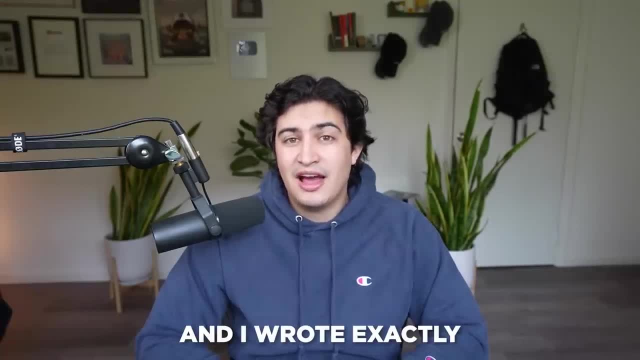 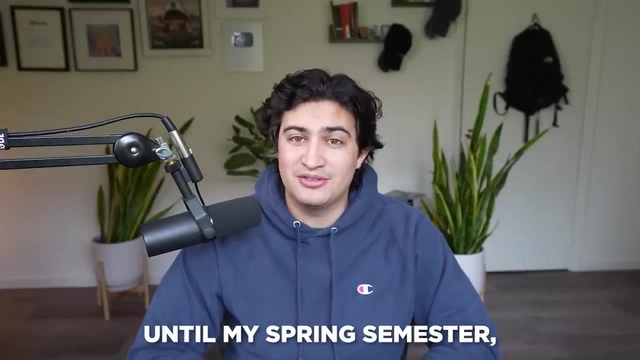 And working hard is okay. Freshman year came to a close and I wrote exactly zero lines of code before my fall semester of my sophomore year. Just kidding, I actually did not write a single line of code until my spring semester's sophomore year, The next class I had to take for my CS major. 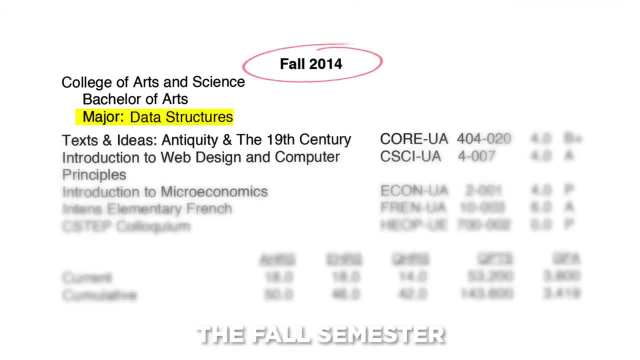 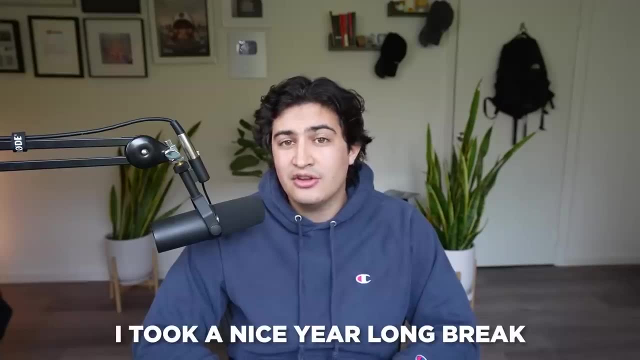 was actually a data structures class and it was offered during the fall semester of my sophomore year. But I didn't take the course then for two reasons: One, that's way too logical and two, I'm an idiot. Instead, I took a nice year-long break from programming and let all the information 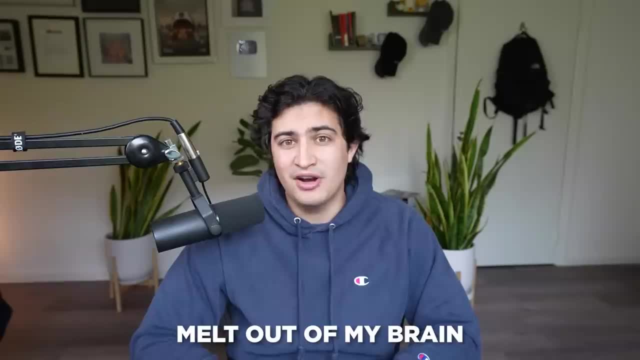 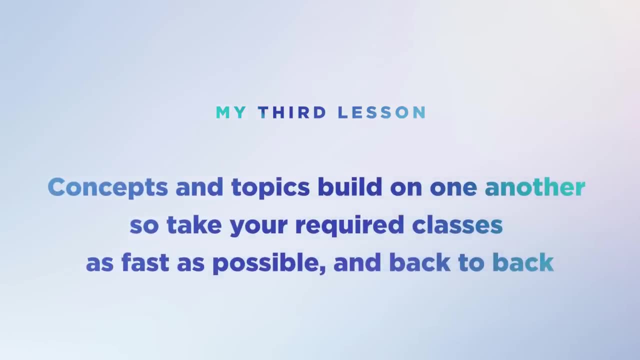 that I somewhat learned during my first year of college literally melt out of my brain, And this was my third lesson that I learned about programming. Concepts and topics build on one another, so take your required classes as fast as possible and back to back. Breaks will break you, And that's exactly what data structures did to me, Armed with 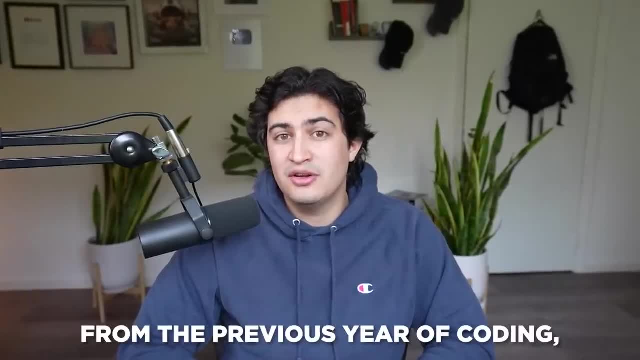 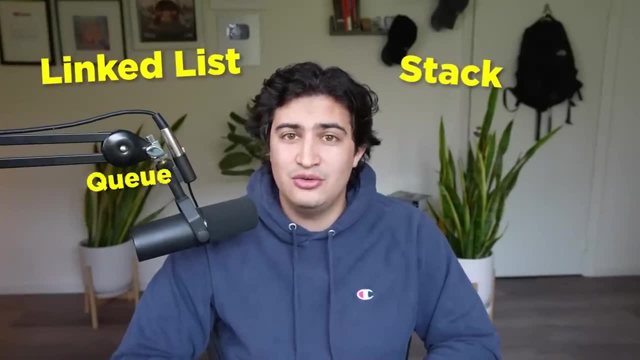 effectively zero knowledge from the information that I should have retained from the previous year of coding. I braved data structures. Once again. I struggled during the class and could not for the life of me create a linked list, stack queue tree or any other useful data. 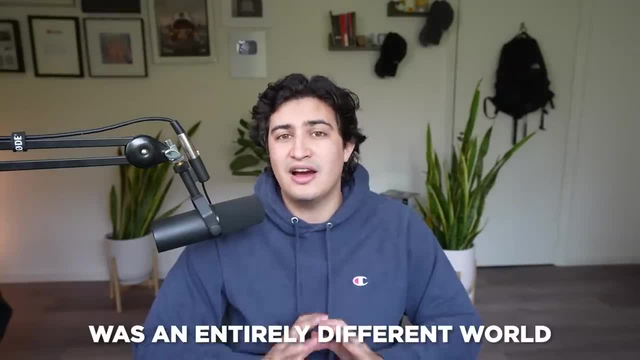 structure. While I had had trouble, the previous two classes- data structures- was an entirely different world. I had never struggled with data structures before. I had never struggled with this much in an academic pursuit in my entire life. While I attended, classes went to the 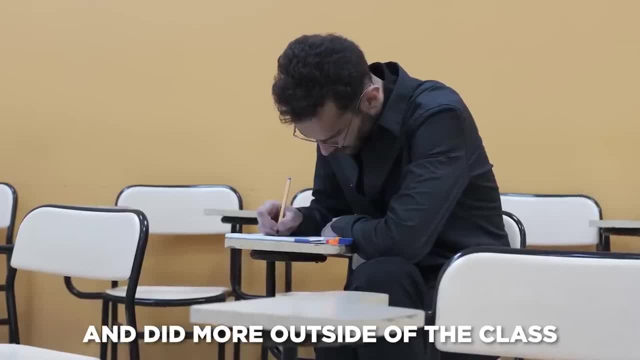 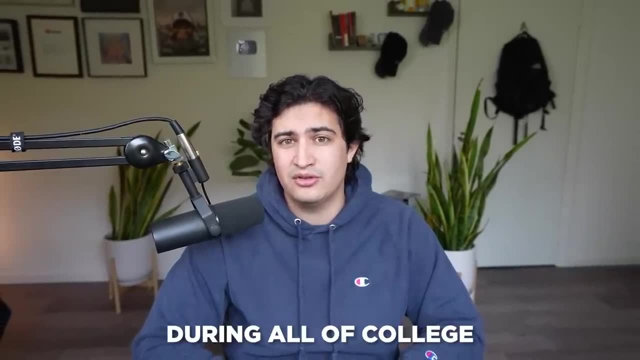 lectures, did all the homework, went to office hours and did more outside of the class on my own. I seriously struggled to grok any of the information I was supposed to learn, and this led me to probably my lowest point during all of college. I remember vividly for one of my data. 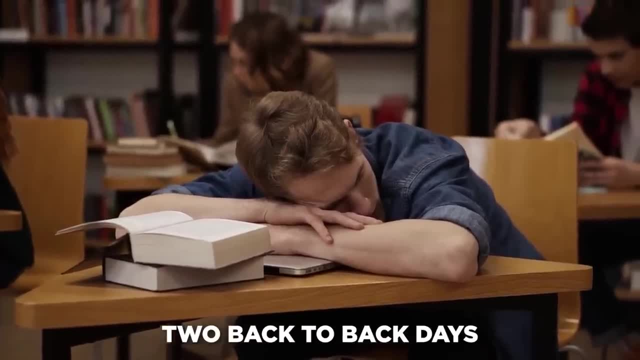 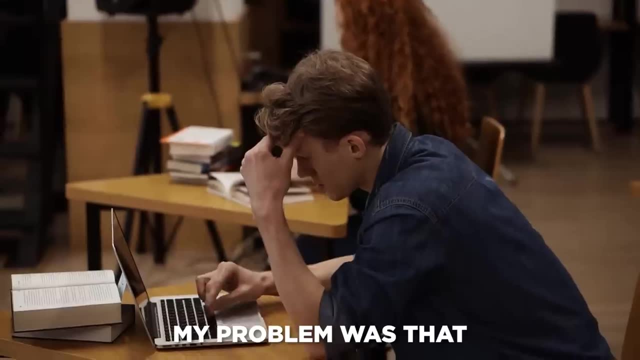 structures assignments. I actually slept in the library two back-to-back days. I know what you're thinking: I probably started the assignment late. but I actually didn't. I started every data structures assignment the day it was released. My problem was that I just couldn't write the code. 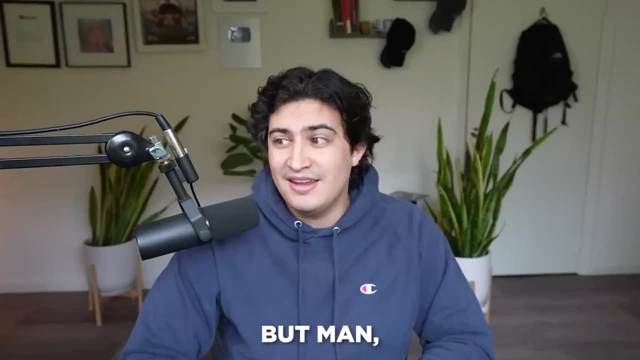 I don't know if you've ever had the pleasure of sleeping in the library to finish an assignment, but man, it fucking sucks. When I studied in NYU's library Bobst, I always studied on the west side of the fifth floor, or as we called it, five west. Bobst has this fun thing actually. 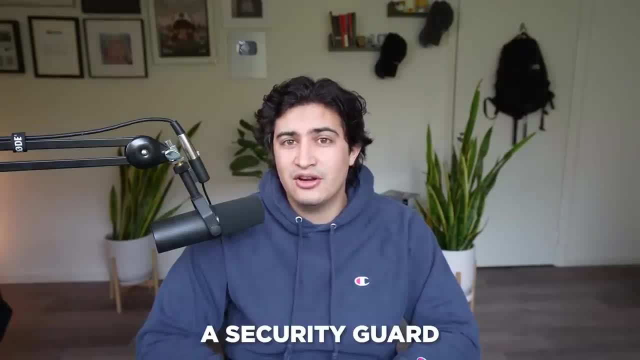 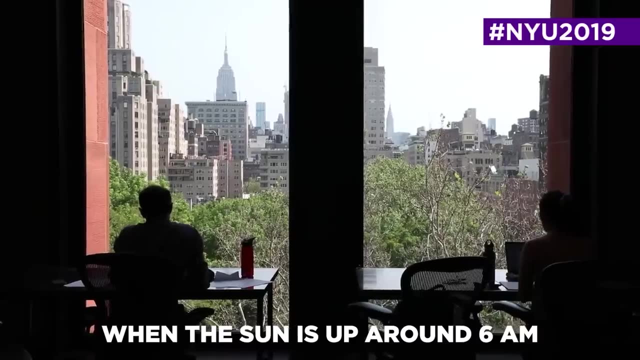 where, at midnight, if you're still unlucky enough to be in the library, a security guard comes and makes everyone move to lower levels one and two. So you go underground when the sun is down and then you come back above ground when the sun is up around 6am, And man, oh man. 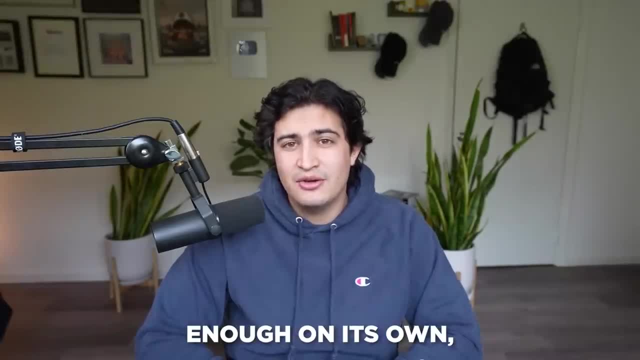 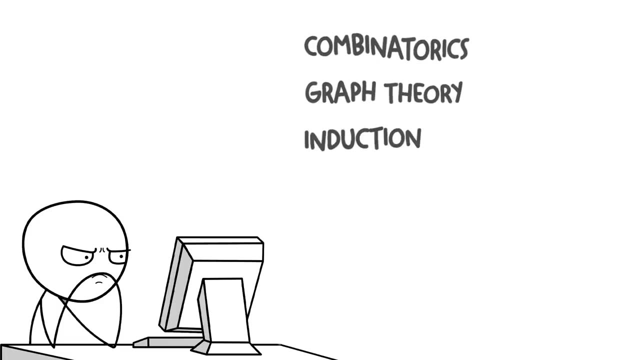 does that fuck with you? And if data structures doesn't sound terrible enough on its own, it was perfectly paired with discrete math, which I was also taking that semester. In discrete math, I learned about combinatorics, graph theory, induction, permutations, Chinese remainder. 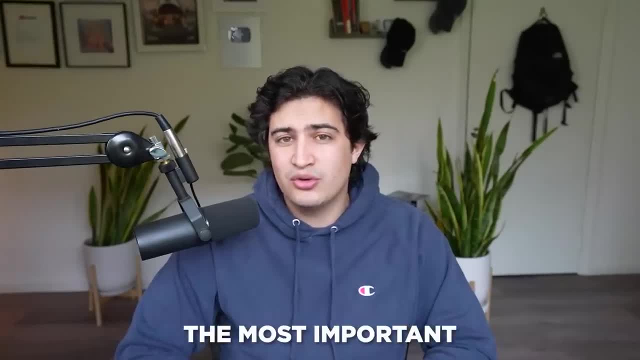 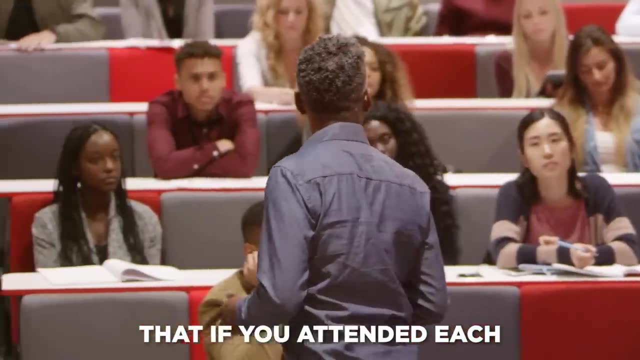 theorem, Eulerian paths and more. But by far the most important thing I learned during that class was how to set an alarm, Because, even though the class was an 8am class, my teacher swore that if you attended each and every lecture he would not fail you, And therefore I dragged my zombie self. 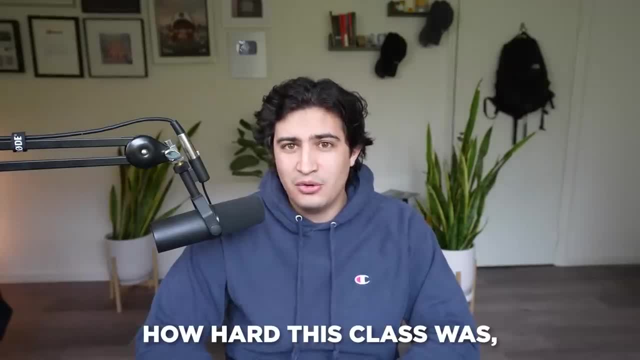 to each and every lecture. To give you just an example of how hard this class was, our teacher actually praised us after our midterm, saying that we all did really well and that we were doing really well. The highest grade on that midterm was a 36.. A 36 out of 100. I think I got. 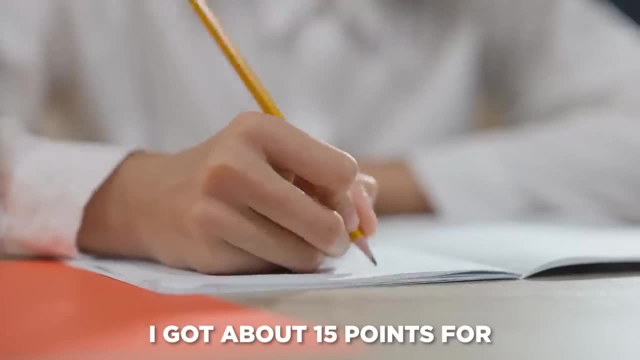 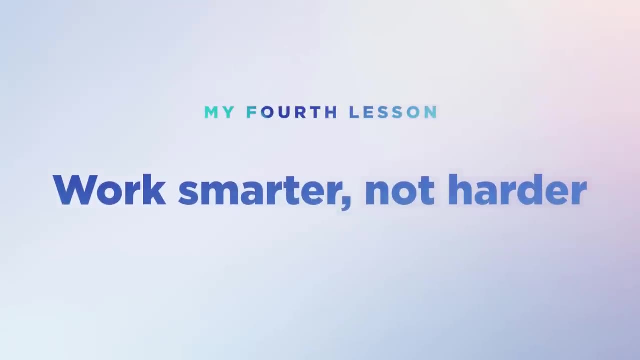 a 24, if I remember correctly, and I'm pretty sure I got about 15 points for just writing my name. And while this semester definitely sucked, it really taught me a lot, most notably two things. First, work smarter, not harder, Just because I was sleeping in the library and putting in tons. 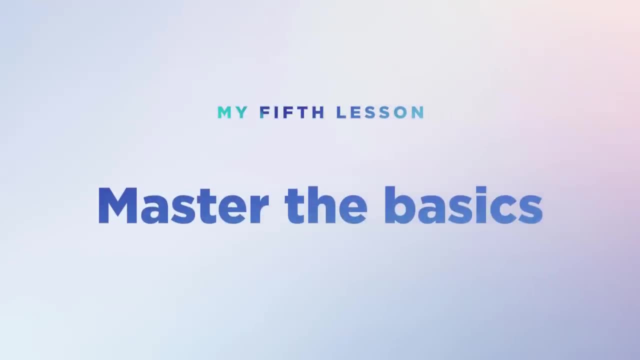 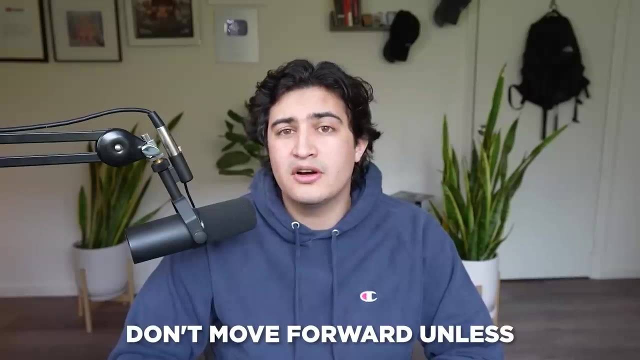 of hours, that doesn't mean I was working efficiently. Second, master the basics. Most of the problems I ran into in discrete math and data structures were because I didn't understand enough about lower level concepts. Don't move forward unless you're a good student And if you. 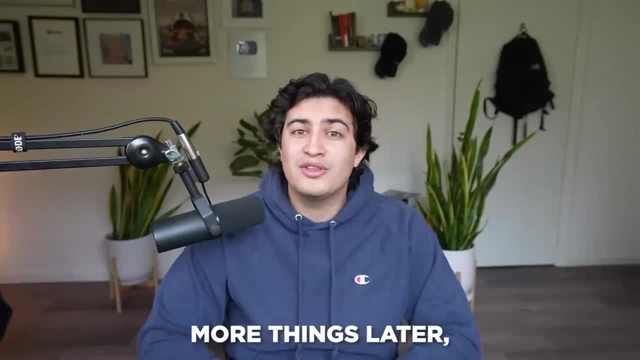 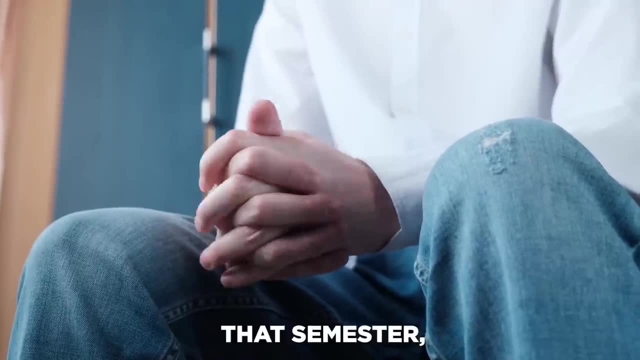 understand something fully, especially if you're going to need that something to learn more things later, which, spoiler alert, is basically always the case in math and computer science. I was super worried about the grades I was going to receive that semester And I needed at least a C in data. 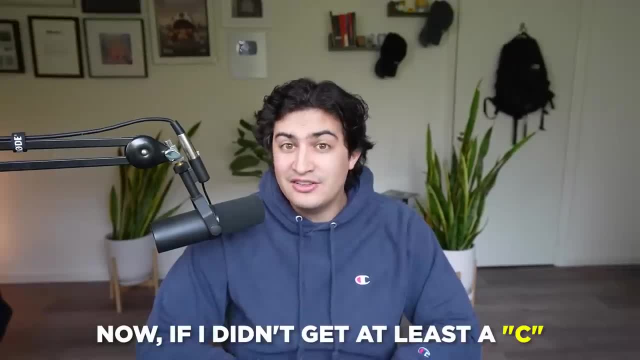 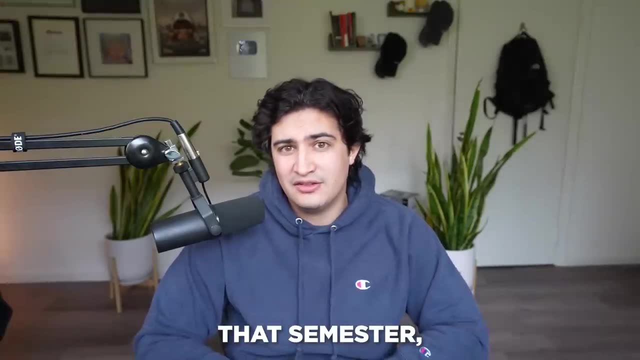 structures and discrete math for that credit to count towards my major. And if I didn't get at least a C in both those classes I would have to retake those classes, Unless I changed my major. I remember right before finals that semester I was reconsidering my major entirely. I vividly 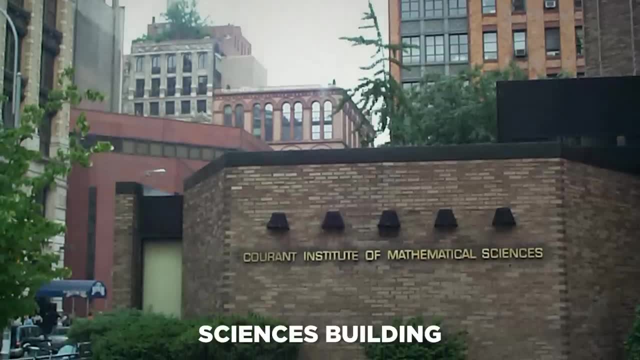 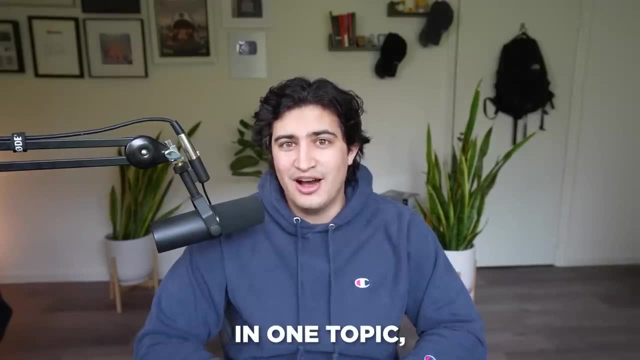 remember sitting outside one of the lecture halls in Courant, the mathematical science building, and literally going through every single major that NYU offered. And after exhausting the entire list and only being interested in one topic- computer science- I decided I had no choice but to. 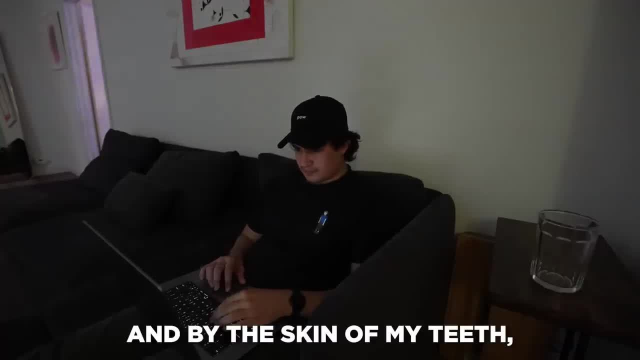 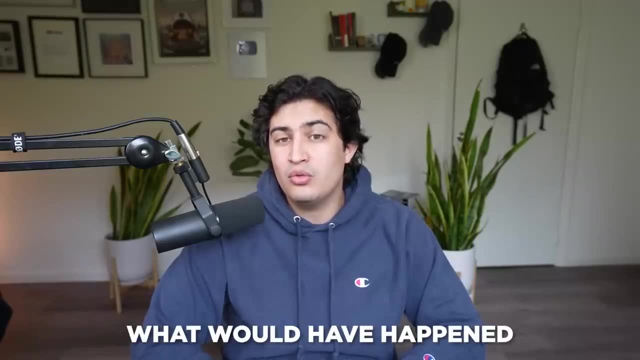 sort of just stick with it. This pushed me extra hard to study and by the skin of my teeth, literally, I was able to get a C in both data structures and discrete math. I weirdly look back at this time and wonder what would have happened if I did end up changing my major 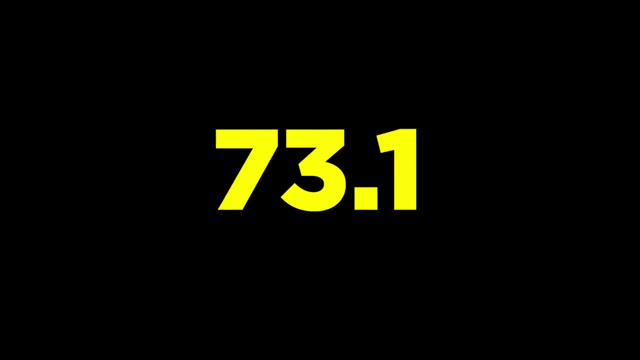 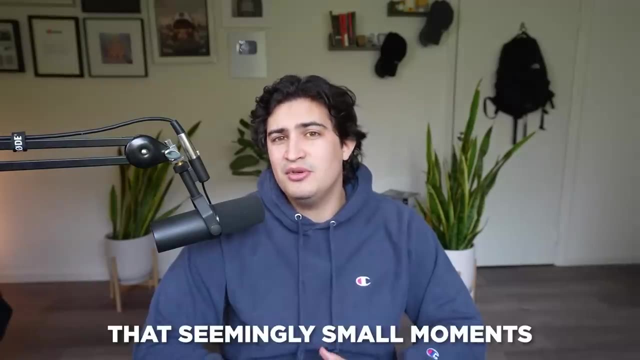 or if I didn't get a final average of 73.12 in my data structures class. That's right, I'm not being dramatic. I really was that close to having to retake that class. It's crazy to think that seemingly small moments can totally change our trajectories in life. and I remember the end. 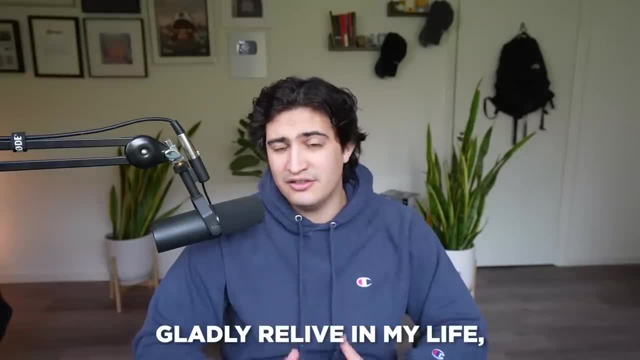 of that semester being one for me. While it's not a time I would gladly relive in my life, it definitely taught me a really valuable lesson. Things worth having don't come easily, and this was definitely the case for me with computer science, But that's okay. 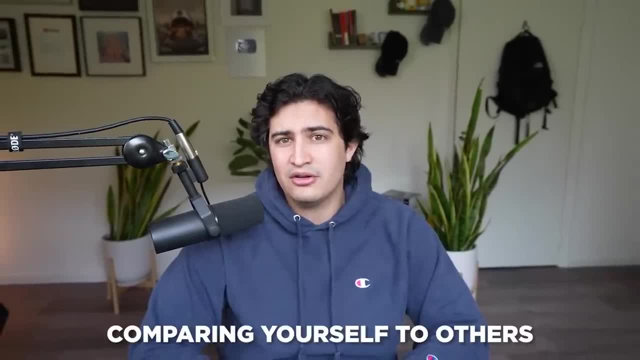 and even though tons of my peers were having no trouble getting their CS degree, comparing yourself to others isn't very helpful. Everyone makes mistakes and learns at their own pace. What's important is that when you make mistakes, you learn from them, And that's what 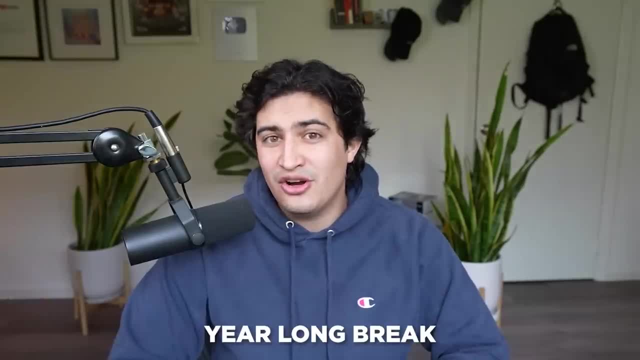 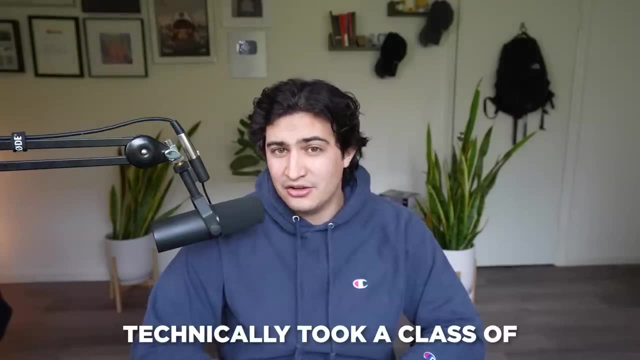 I didn't do when I decided to take another year-long break from coding classes and run away to London to study abroad. I was now in my fall semester of my junior year, all the way in London, and while I technically took a class of linear algebra, that did count as a computer. 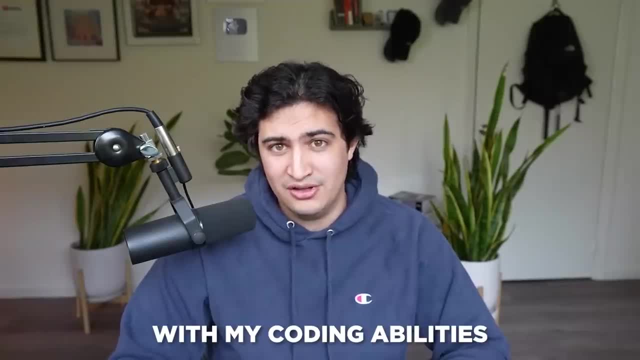 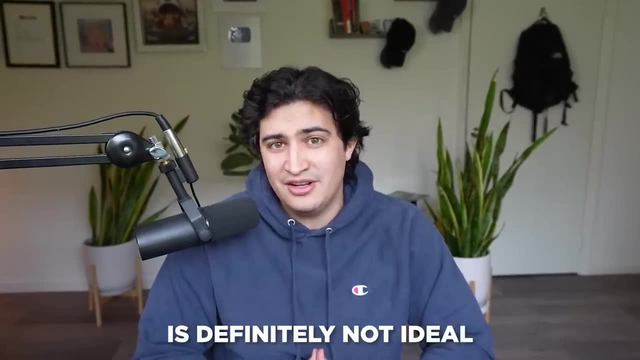 science elective, it did not help me at all with my coding abilities. Looking back now and knowing that everything worked out, I don't regret going abroad, but taking long gaps between coding classes specifically is definitely not ideal. While abroad studying linear, I learned about 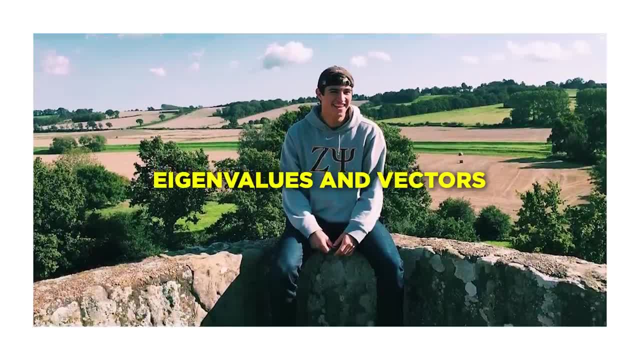 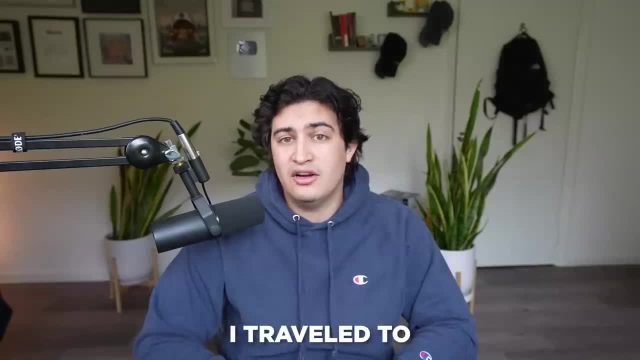 matrix, multiplication, reduced row, echelon form, eigenvalues and vectors and, most importantly, that British people call math maths and that they refer to zero as not. When I wasn't in class, I traveled to a ton of different places like Edinburgh, Glasgow. 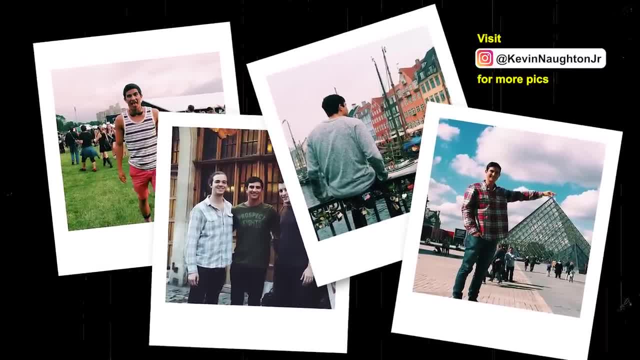 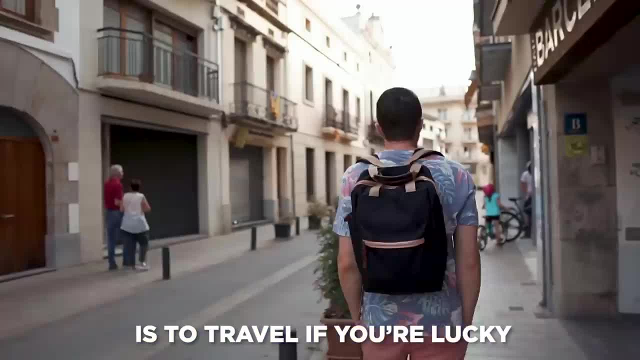 Copenhagen, Venice, Florence, Rome, Prague, Munich and more. It was a great semester and I really appreciated that I was able to go live somewhere else in the world and learn about other cultures and ideas. The lesson I learned here is to travel if you're lucky enough to be. 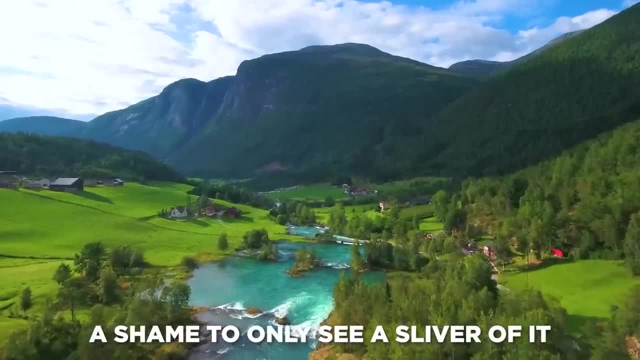 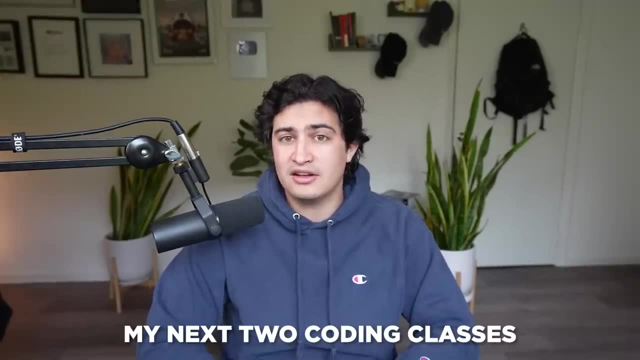 able to. The world is an incredible place, and it'd be a shame to only see a sliver of it. The semester was over before I knew it and I headed back to the United States with my B-plus in linear algebra and my new vocabulary and I prepared to take my next two coding classes. 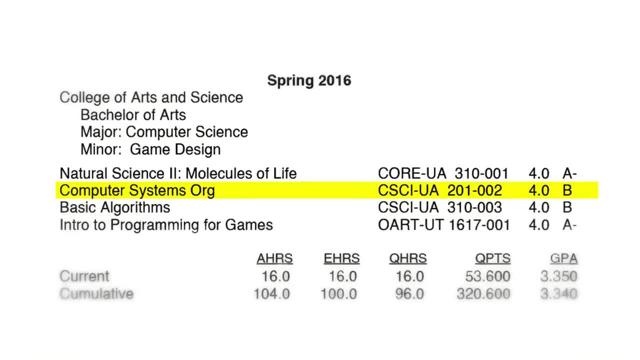 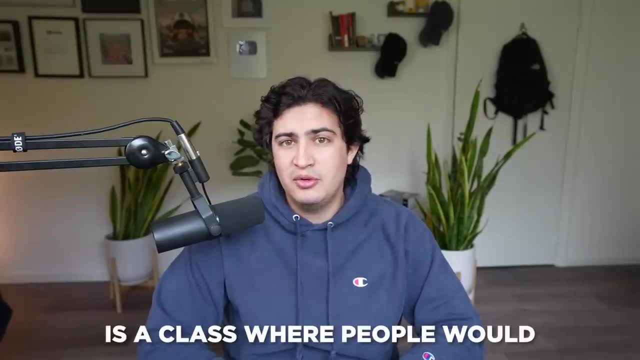 during my spring semester of my junior year- CSO- Computer Systems Organization and Basic Algorithms- And these were two of the hardest classes for the computer science major at NYU. People always said that CSO was a class where people would decide to continue with their degree. 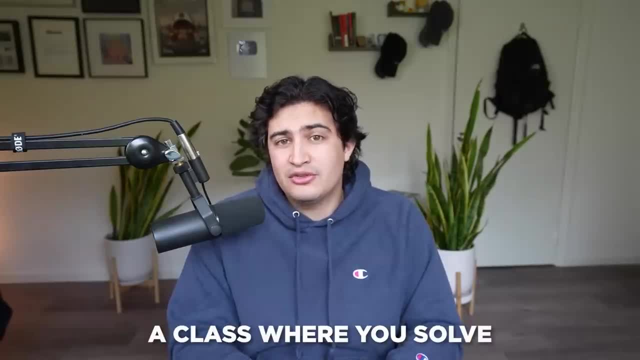 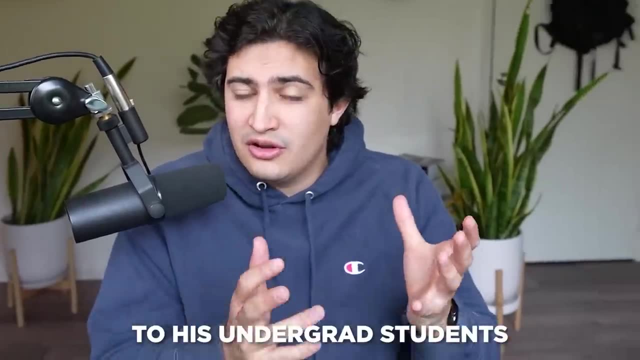 or just bail out with a minor At Basic Algorithms, a class where you solve strange riddles and mathematically prove their runtimes using widely researched techniques, and a teacher who likes to assign his grad students homework to his undergrad students. and I was all but sure I 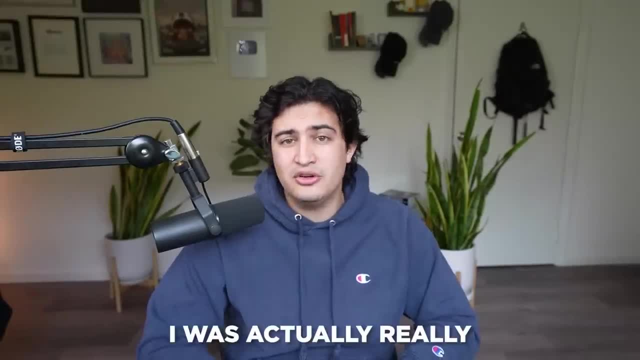 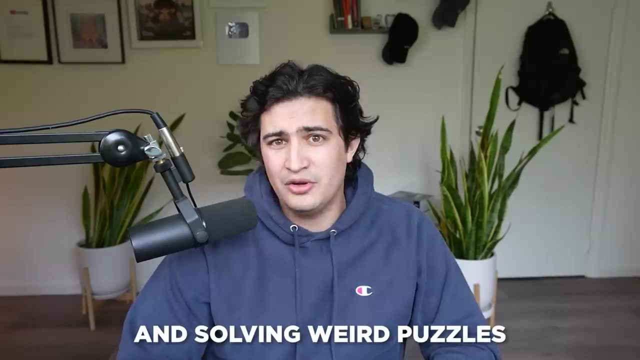 wasn't going to fail But to my surprise I didn't. And, even stranger, I was actually really enjoying learning about lower-level topics like bits, pointers, memory caching, concurrent programming and more in CSO and solving weird puzzles and algorithms. And while these classes 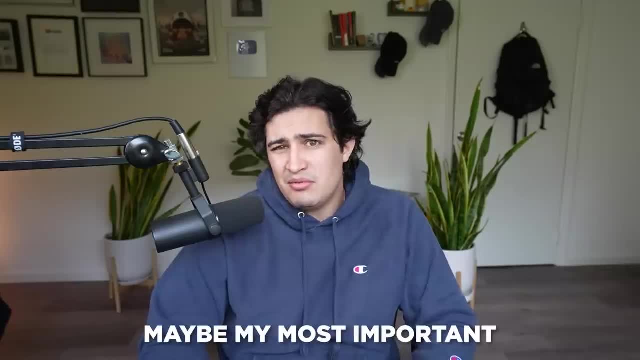 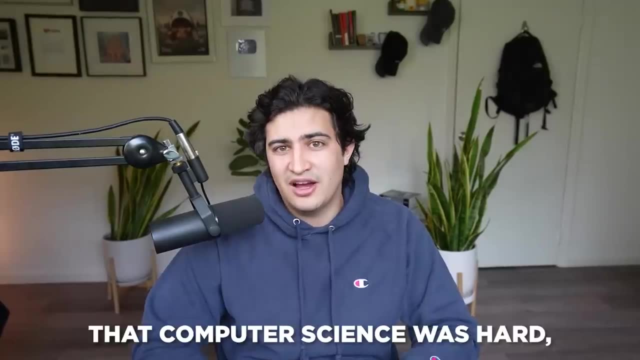 were hard, I was able to do them and I was shocked, And this taught me maybe my most important lesson. yet Most of the things I found hard were because people or society made me think I was supposed to. People would tell me that computer science was hard and therefore I would. 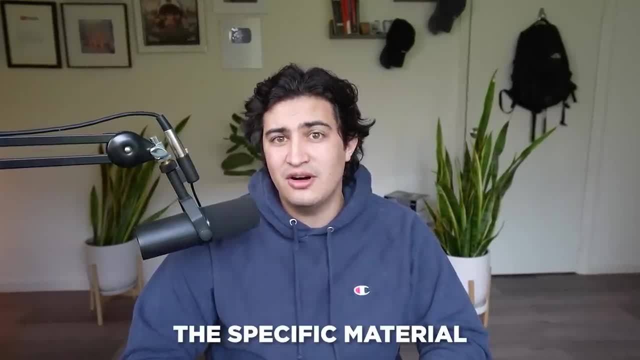 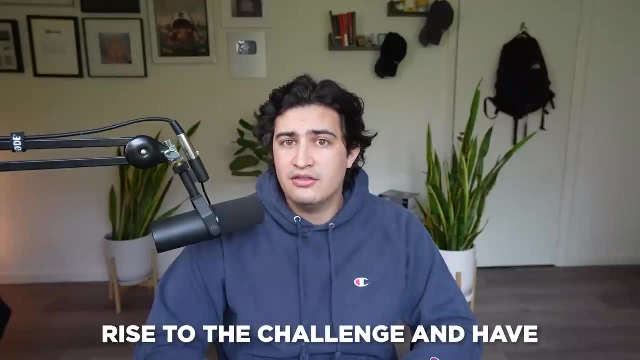 think it was regardless of how I actually felt about the specific material I was learning at the time. Don't do this And instead come to your own conclusions. If something is hard, rise to the challenge and have confidence in yourself. You can figure out almost any problem with enough time and effort. 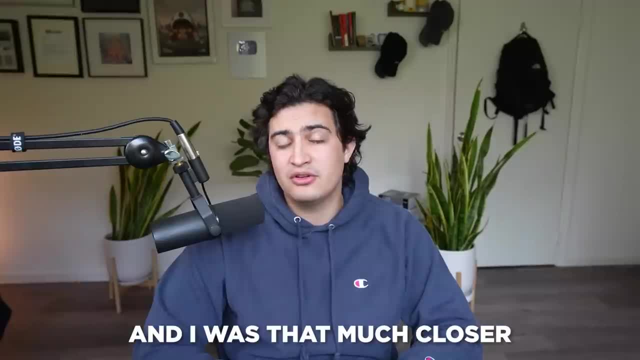 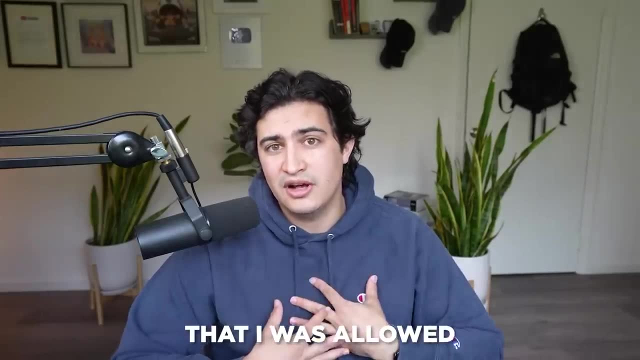 The semester flew by and I received Bs in both my classes and I was that much closer to finishing my CS major. All that was left was one core class, operating systems- and three computer science electives that I was allowed to choose Over. my next and final year at NYU, I took 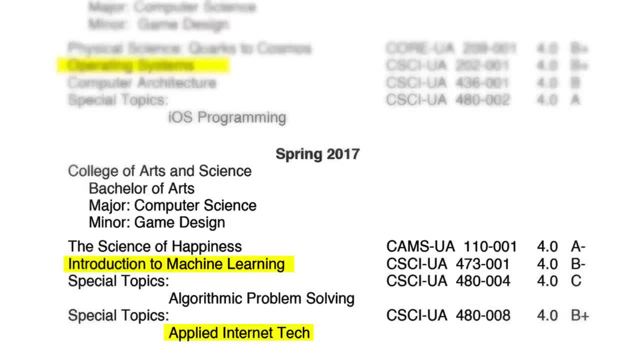 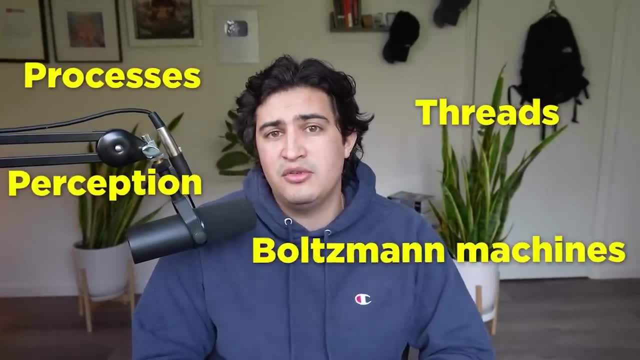 operating systems, intro to machine learning, applied internet technology and algorithmic problem solving. I learned about so many different topics in each of these classes, like processes and threads, perceptrons and Boltzmann machines, full-stack web development and how to pass coding interviews, respectively. This was probably my favorite semester and it was 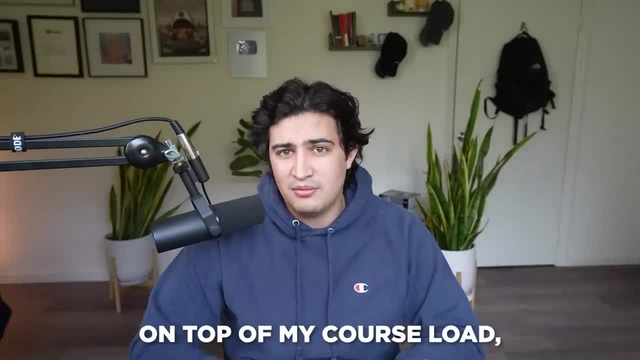 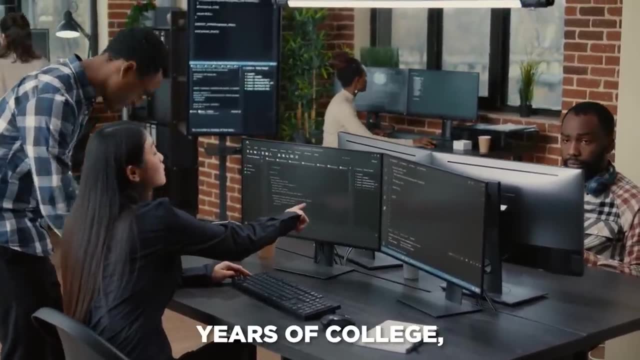 crazy to think that college was coming to a close. Throughout the entire semester on top of my course load, I could not stop thinking about finding a full-time job. Lots of people I knew actually had internships in computer science throughout their years of college and a lot of 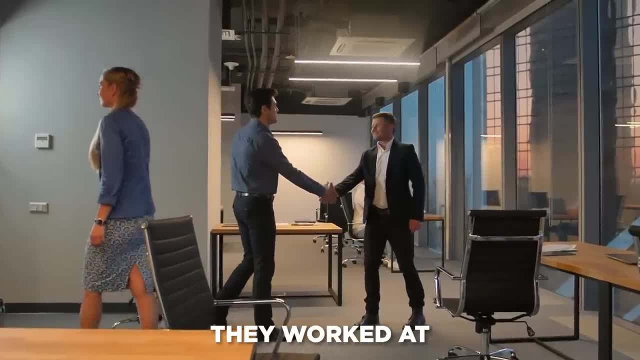 them had already decided to sign full-time offers from the companies they worked at prior to their senior year. Luckily for me, algorithmic problem solving was the perfect class because it prepares you for the kinds of questions I had to ask myself. I was able to do a lot of the things I wanted to. 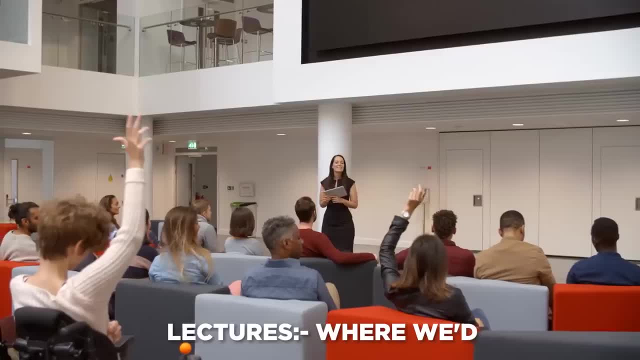 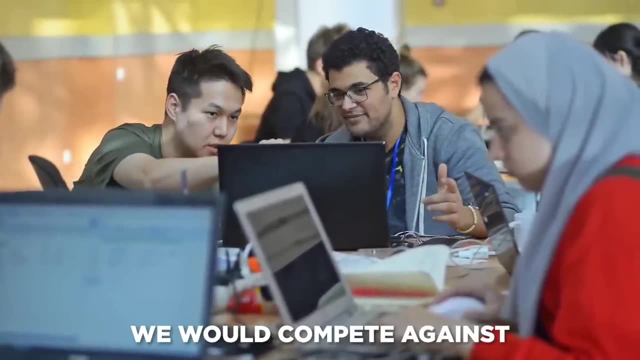 be asked during coding interviews. The class consisted of two components: lectures, where we would learn about algorithms and how to write code to apply them to real-world problems, and coding competitions, where every Friday live, we would compete against one another to solve a problem.